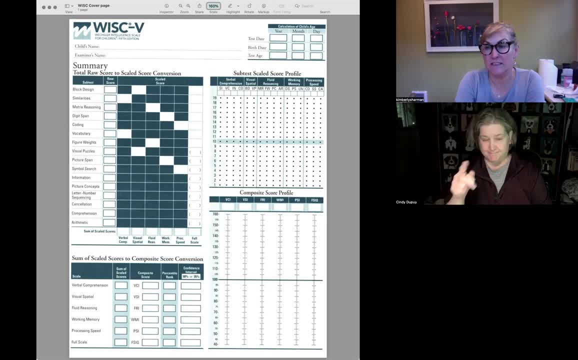 Well, you can't take it home, but you can sit in a room in the school and look at the raw protocols, which is the data from your testing. Yes, And there's actually some debate as to whether or not you can take the protocols home. 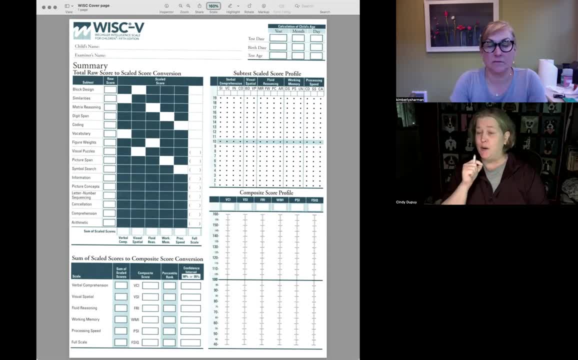 But let's not push too many buttons. Let's just say that you actually go in and you want to look at this protocol, And so a couple of things you should first check for- And the biggest one is right here: your child's name and your child's date of birth. 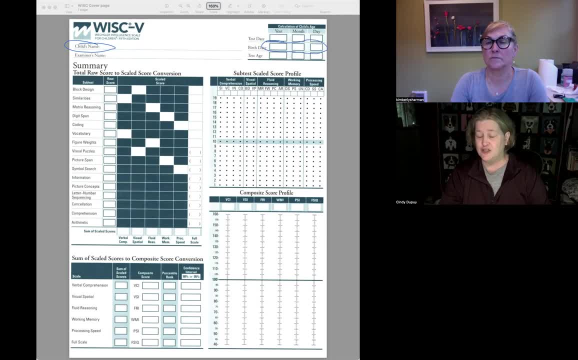 And make sure that you've got the right protocol. I know that sounds super simple and stupid, but you're going to let your child test different schools. I know I'm saying this because I've seen different students names inside reports, which leads me to believe that. 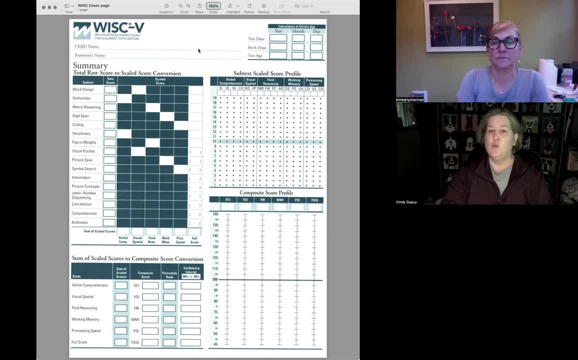 Sometimes clinicians make mistakes because they have too many people and they're trying to do too much, So anyhow. so that's the first piece. now, When we start navigating the protocol, this summary area is kind of the most important thing. Now, Kim, you see what it says, Right? 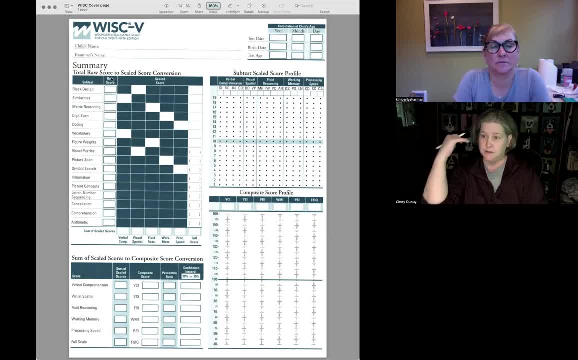 So your raw score is where you've totaled up the individual scores on each of the items on the test. OK, so then, as a clinician, I would come in and say, hey, this kid scored a 34.. On block design, they scored 27 on similarities. 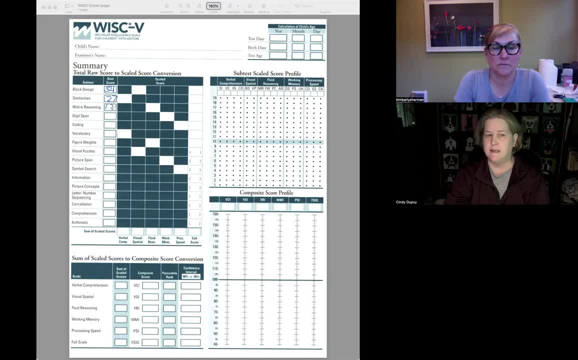 I'm just randomly making up these numbers. Let's say they got an 18 and so forth. So, as we put in these numbers, this is what the clinician would then use to go in and look up on norming tables to find out how this converts. 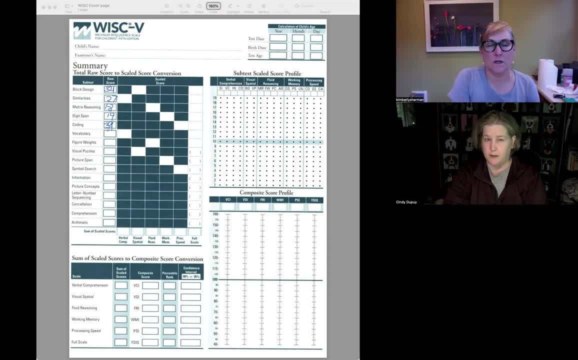 Does that make sense when I'm explaining it to you that way, Kim? Yeah, So these norming tables. and when you say it converts, what is it going to convert to? So the raw score Converts to, initially, a scaled score based on your child's date of birth. 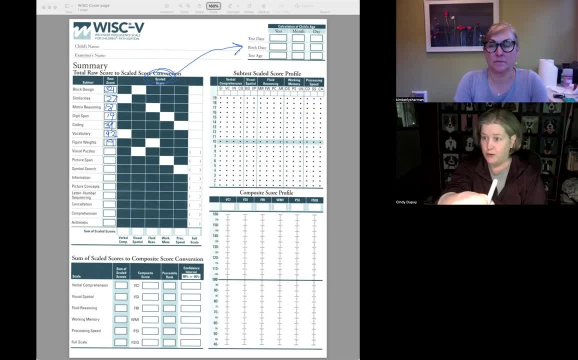 Now, if you happen to look at this protocol and you see that your child's date of birth is wrong, That is a major red flag. OK, something has gone terribly wrong, And I would encourage you to reach out to a professional outside of the school district- a clinical psych who administers these things- and have them review the protocol for you. 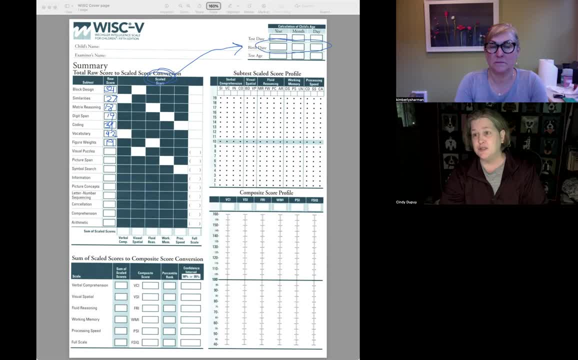 But don't necessarily go straight in and call it out to the school district At the get go because you want- You want to see the document in its original state, to have somebody independently review it. That would be my suggestion to you: have somebody who is not associated with the school district. 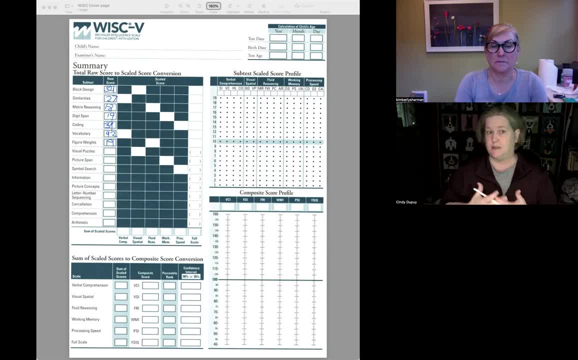 Get a copy of the protocols. The district can send them to that clinician. have them review the protocol to see if things were done correctly. OK, because that testing age here tells us what table to go and look up the norms. You know what I mean by norms. So, yeah, your scores are going to be all messed up and what you're comparing- the raw scores- And what you're comparing the raw data to is going to be incorrect Because you've got the wrong age. That's right. So when you're young, a shift of a month or two 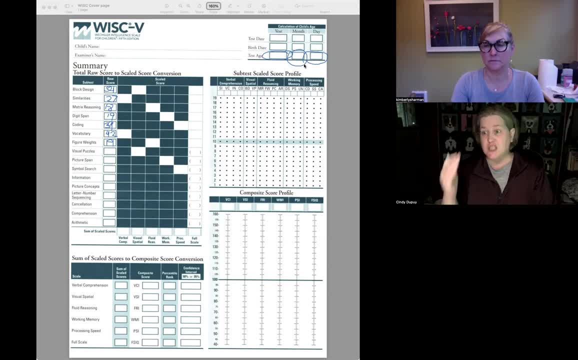 Is a big deal. Once you start hitting 12,, 13,, 14, then you're looking at six months. But if somebody didn't get the date of birth right, I would still want somebody going to look at the protocol. I just would. 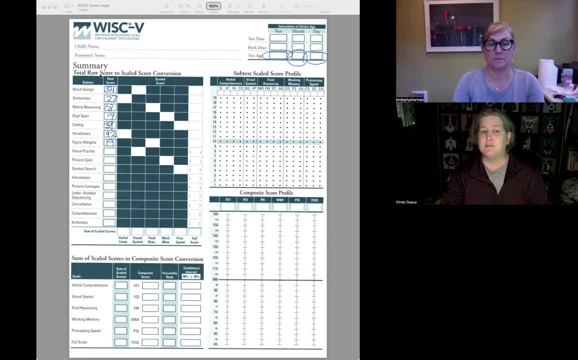 OK, this is a real basic, OK. so then I go into this miraculous Table and I would say, hey, let's, I'm just going to randomly make up these numbers and they are likely not going to be correlated to this at all. 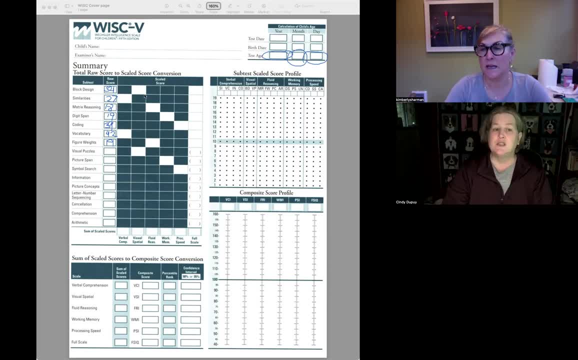 So I'm not comparing this to any norms, I'm just making up numbers. Again, this is a special book that the testing administrator has that re-evaluates these numbers, Right. So I go in and I say: hey, you are 12 years, seven months and 18 days old. 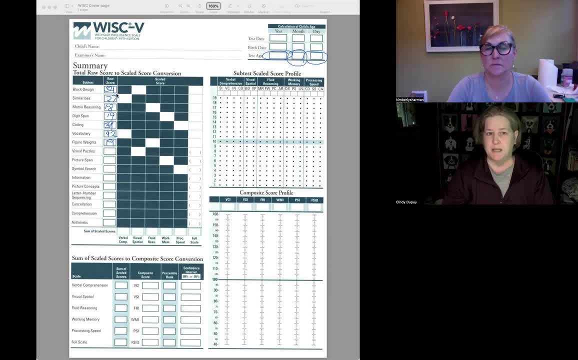 Here's my table. When you get a raw score of 34.. On block design, that means you have a scale score of 12.. Now I've done- we've done a little blurb on what are scale scores, standard scores. 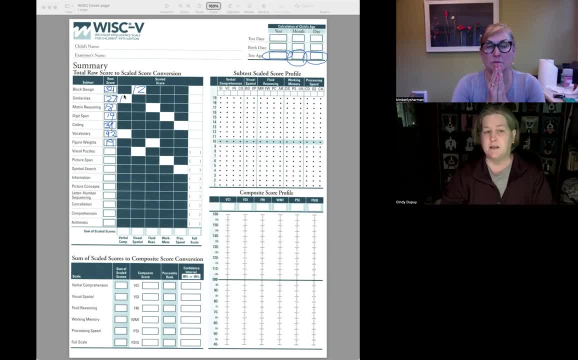 So bear with us on that. Let's say, on similarities, you've got a 13.. Let's say on matrix reasoning: you got a seven. Again, I manage miraculously just making these numbers up. Coding at a 39 is going to be incredibly low vocabulary. 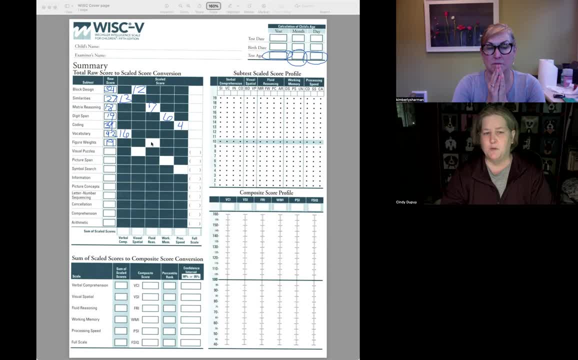 We're going to make that a 16. just to make it interesting, Figure weights- we're going to call that also An eight. we're going to give that as low. And then we didn't do visual puzzles. Now do you notice right here, Kim, that we have a column of numbers? 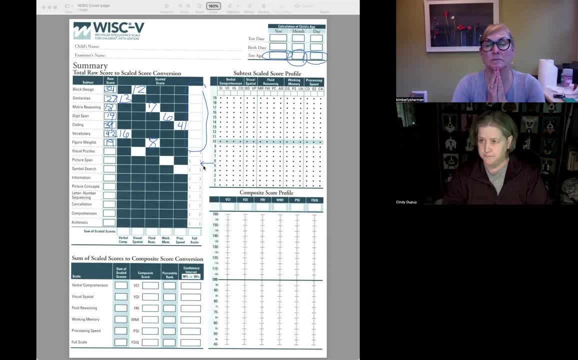 that don't have these little parentheses around them. Yes, Are you wondering what these little parentheses are for? I think those are the alternate tests that you can use Over the years of being around me. So let's say, you go in and you do. 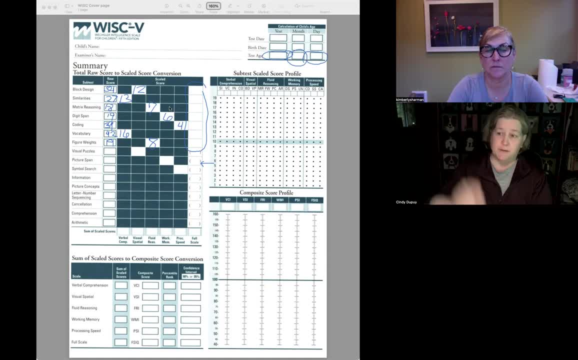 Matrix reasoning. and in the middle of doing matrix reasoning you have a fire drill. And I shouldn't say matrix reason. Let's say you have a fire drill in the middle of block design. There is no way you're easily going to be able to recover that score, because if the fire alarm went off right in the middle of a student finishing a puzzle, it's going to throw off the time. 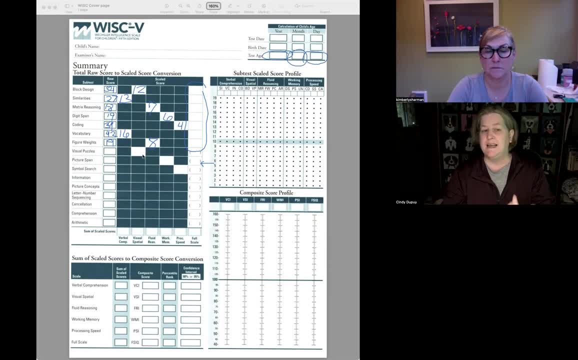 So at that point you have to substitute a different subtest, You have to take the place of that, And so a lot of schools are still giving all 10 subtests of the WISC, And so those scores may be provided, but it doesn't necessarily mean that they're calculating the full scale IQ. 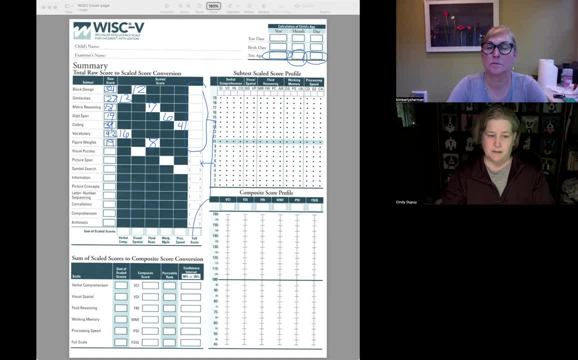 So these seven scores here come down, and I'm going to pardon, I'm going to draw a really bizarre line all the way down here. The sum of those is what gives you the full scale IQ. Okay, All right, So now do you know? 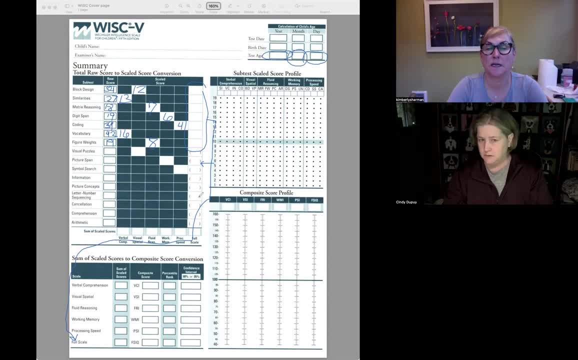 First, we have columns here where there are two boxes in each column. Yes, Okay, We are going to add those two numbers up and we're going to use them. I'm going to get rid of this very long line here. We're going to use them to calculate the index score. 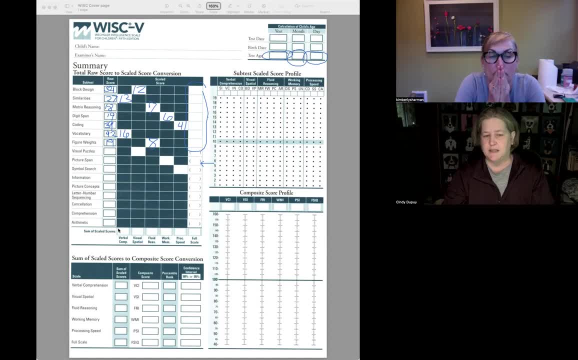 So we have 13 plus 16, which gives us a 29.. And it does help if I regrab my drawing tool. So we've got it. We've got a 29 there, okay. Visual spatial: give me a number for visual puzzles. 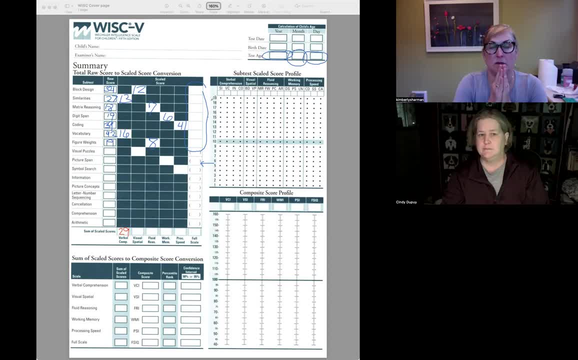 What number do you kind of want? Oh, I don't know, 15. Okay, Let's say they did incredibly well on that And let's call picture span something low. Let's give it a four, and then we're going to give symbol search a five. 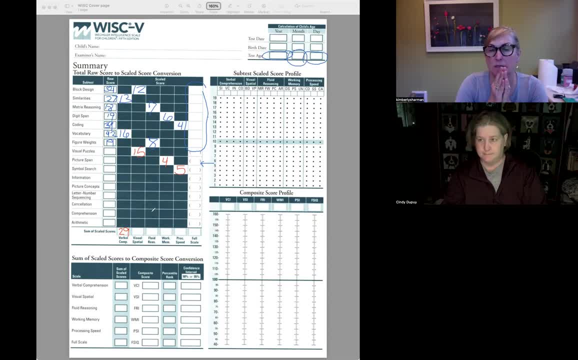 And that'll make more sense. Is that also something to be wary about? if the subtest that could substitute for it Is that different from the other one? Yes, Each subtest is different and is used for different reasons, and there are particular options. 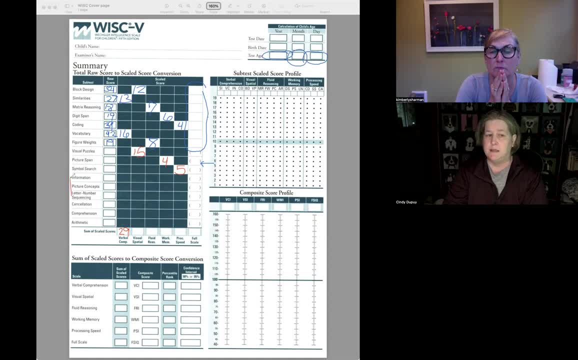 So, for example, letter number sequencing substitutes for digit span or for picture span, but not anything else. Cancellation substitutes for symbol search or for coding whoops, but not anything else. I assume it's not just a four, It's a fire drill that would make you go to a subtest. 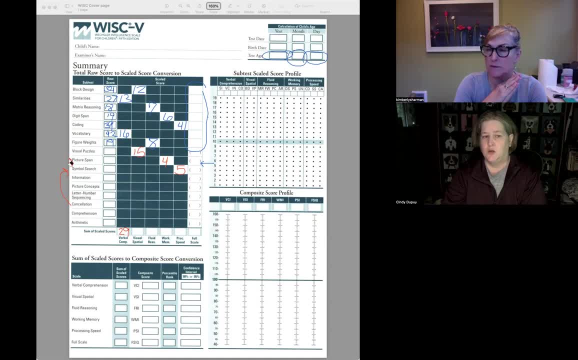 What are other reasons why they would go to a different subtest, these additional ones? So I will occasionally make the decision to, in advance of administering the test, say, I do not think that this student will do particularly well on this test for X, Y, Z reason. 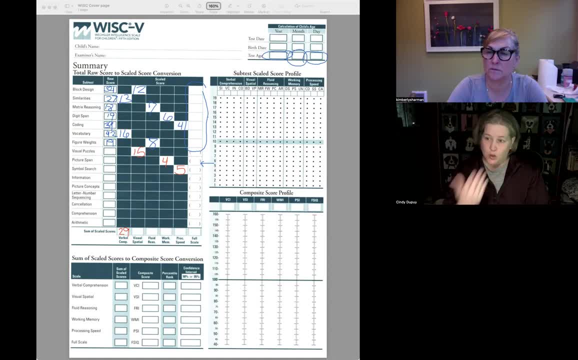 So I have students with oral language issues. like they have a hard time expressing their ideas and similarities and vocabulary could be really difficult for them. Information is more of a point on do you have a piece of factual knowledge or not. It's untimed. 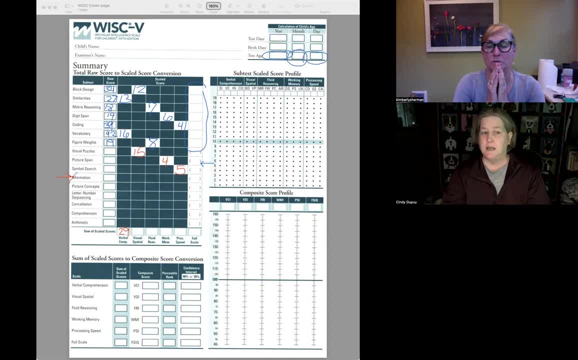 You can take as much time to get your answer. Sometimes I will choose to substitute information for one of these other verbal tests for a very specific reason. Sometimes I will go in and administer additional subtests Because there are some additional enhanced index scores. 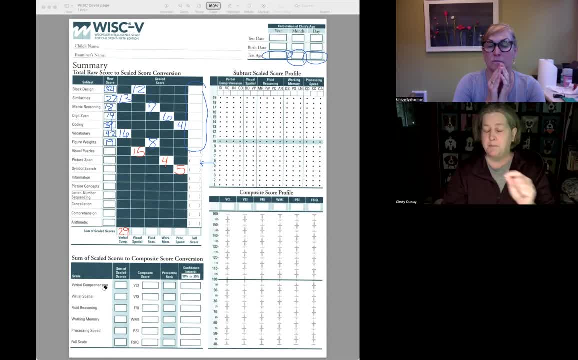 So, for example, while we have a verbal comprehension, there is also- not to confuse everybody- a comprehensive verbal index score which combines similarities, vocabulary, information and comprehension together. Essentially, you use your a lot of times. you smell that this test is very hard. this whisk on kids with dyslexia. 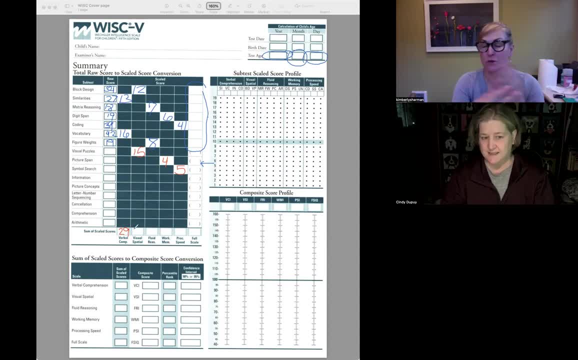 or different extreme, you know word retrieval issues or whatever. So you, you are picking these subtests to show what their true intelligence is, so that you can extricate the extreme learning issue, Yeah- From always going in and digging hard to try and find what I think is happening and why. 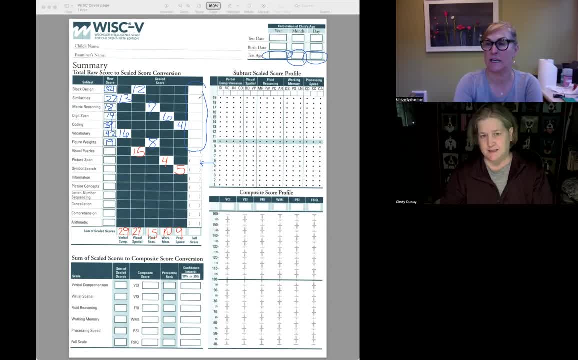 Okay, And they don't really do that in the school district. This is like for outside testing. that will put this extra effort towards that. So you will occasionally run into clinicians who are better trained, who are in the public school system, who know a little more. 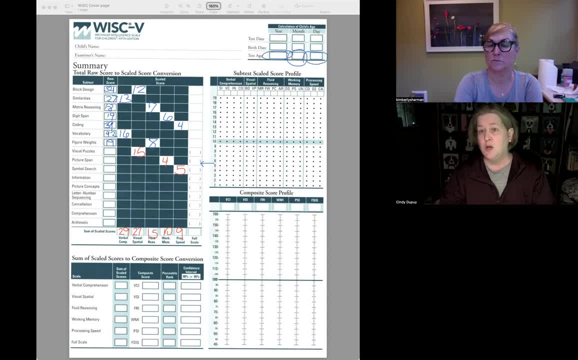 differential diagnosis. but that's not necessarily the norm. Most individuals, most clinical- sorry, most school psychologists- have a master's degree. So that means you've done two years of post bachelor's degree work in administration, scoring those kinds of things. 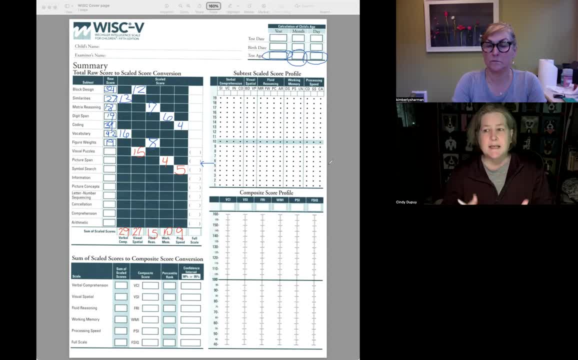 You've had clinical supervision And but you, you haven't necessarily done the deep dive into differential diagnosis the way that somebody who's specialized in neuropsychology would. Does that kind of make sense? Yep, Yeah, It's a different ball game as far as the level of specificity and 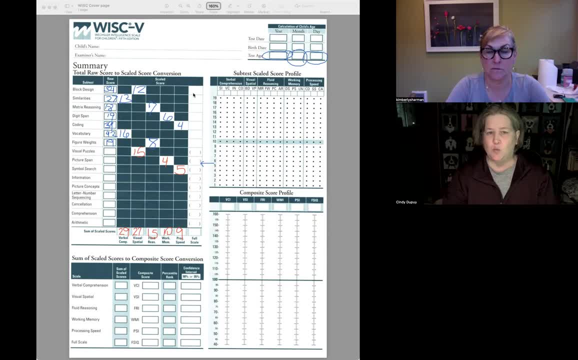 Yeah, Okay. So let's go back in. I'm going to, we're going to add up here. I'm going to put: that's a bad color. Let me change that color one more time. Let's go something. Let's put it in black. 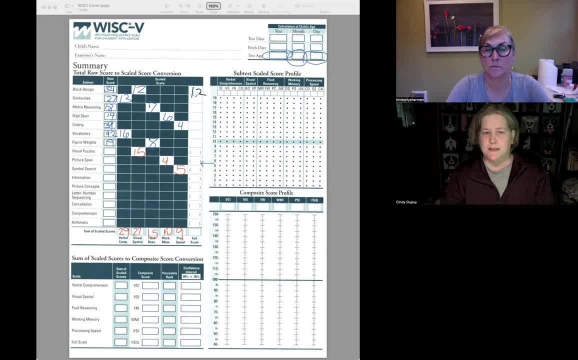 So, remember, we're going to add up our 12 and our 13,, and I will tell you- I always do running totals in my head, just because that's the way that I think, And so let me write down our numbers here. 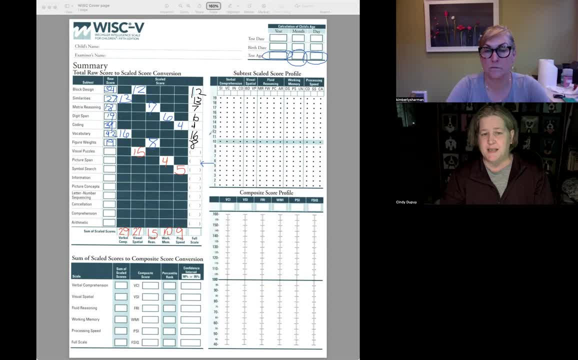 And, by the way, if you see this profile where you have a kid scoring in the top 2% of the United States on one sub test and scoring down in the like third percentile on another sub test, That is a red flag that something else is going on there. 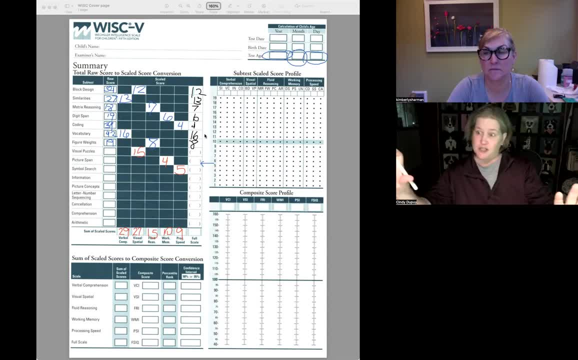 Okay, Which is the difference between the full scale IQ and GAI, which is another one of our videos. Okay, So if we do a little bit of math here, let's see That's 30,, 42,, 50.. 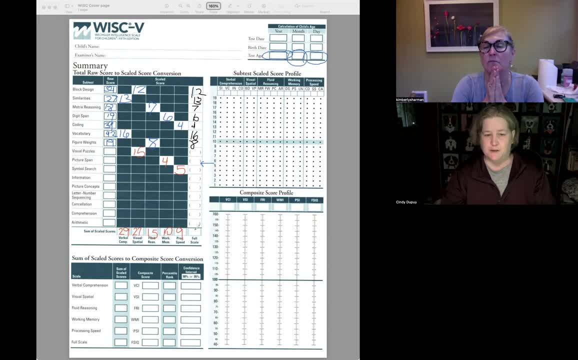 We have. 66 is our total. So our full scale IQ would be based on 66.. Okay, So then we come in down here and we write. We write in our numbers. So our 29 for verbal comprehension goes right there. Our visual spatial is a 27.. 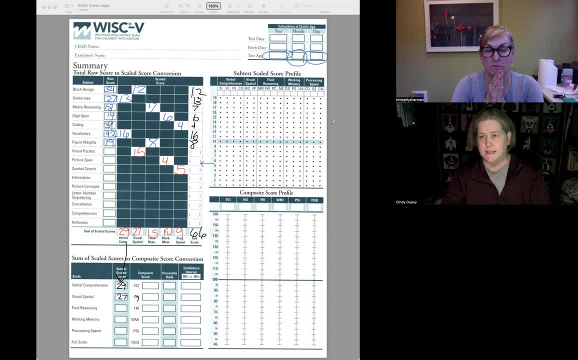 And they have these little abbreviations here to help people kind of track what's happening in each column. Now our fluid reasoning is not very not as strong. So that's at a 15. Our working memory is really a challenge, So that. 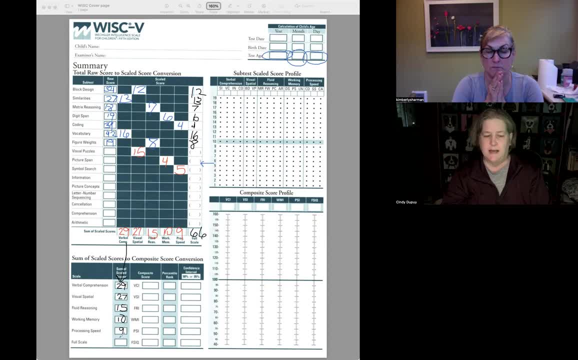 That's a 10 and our processing speed is a nine and our full scale IQ is a 66.. So we've looked up, we've converted our raw scores to scale scores. We now total, we subtotal our scale scores. Okay, We subtotal the seven for the full scale IQ. that gives us the number down here. 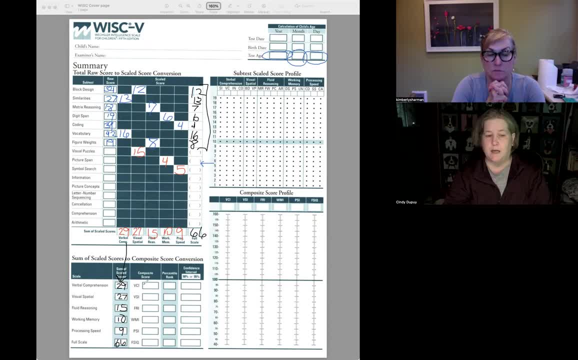 And then we've totaled these down here now at a 29. So we're down by 7. And then we've totaled these down here at a 10. And we subtotal these down, let's say, at a 16 and a 16.. 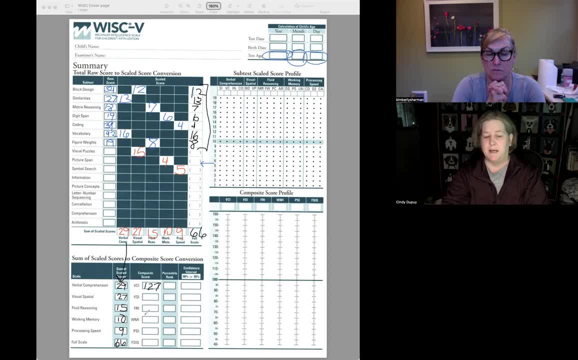 And then we subtotal these down to a 29.. And then we subtotal these down to a full scale IQ, which is a 16 at the top. And then we subtotal these down to a 24.. And then we subtotal these down to a 16.. 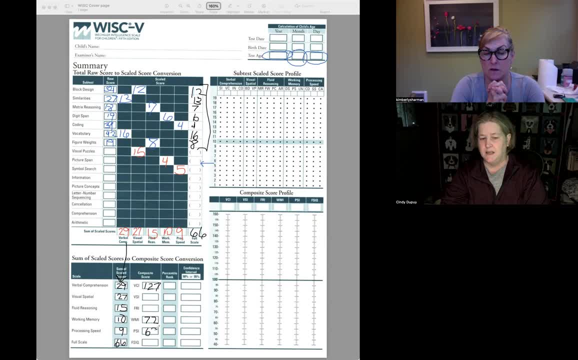 So the total number of count is gonna be about 26. So You're gonna be able to, On verbal comprehension, You're gonna be about a 1: 27.. And that's is so important is that you're looking at a different column in this book based on that. 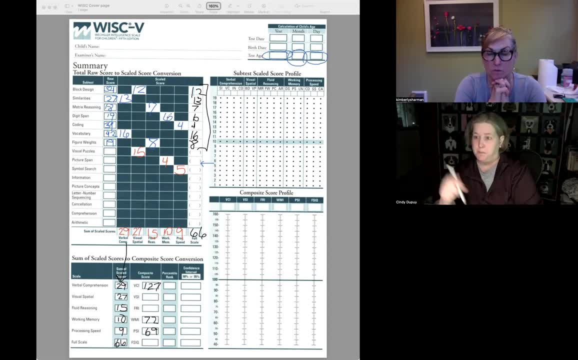 information in the right hand corner, right that data changes by age, so what you're expected to do as you get older is significant, and your scores are supposed to continue to go up. so, um, that's how they create these index scores. um, for the various subtests. now the other thing that should be: 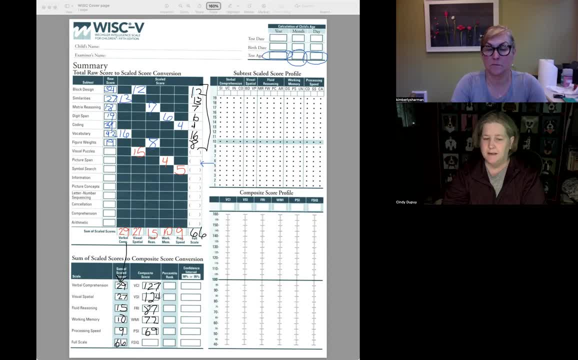 happening. that is frequently not happening- is the clinician is supposed to come in and say: does this make sense when we think about this kit? so you have these wonderful profiles over here, which I never use because I look at the numbers and I think in numbers. okay, but let's go in for a minute and let's mark. so we've got our 12 for similarities. 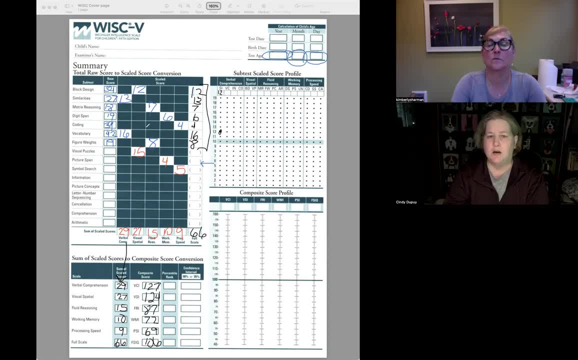 and, and we've got our 16 for vocabulary, And so you'll notice, I'm putting in these little dots. Now, have you ever seen these before, Kim? Have you seen this? Okay, So then they would connect those dots and they would say: hmm, block design is a 12. So let me put a dot there. And visual puzzles. 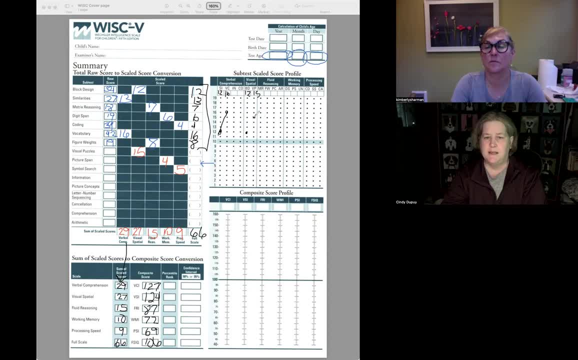 is a 15.. And so I'm going to put a dot there for fluid reasoning. We have got a seven for matrix reasoning And sorry, I'm not writing beautifully given the size and I'm doing it with a finger on a trackpad. Let me see if I can clean that up just a tad bit. So we have visual puzzles was a 15. 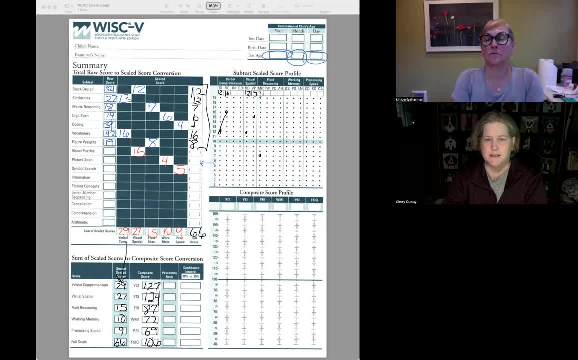 and I really should just type them in Matrix. reasoning was a seven, Figure weights is an eight, Digit span is a six, Picture span is a four, Coding is a four And symbol search is a five. Okay, So you'll notice now that I'm drawing lines between these various 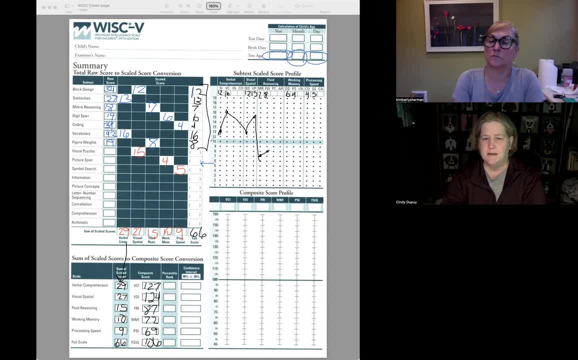 subtest scores Now smack here at. 10 is average Okay, But when we go in and we start graphing this, anybody who has done any significant work in the field, who's done anything on any level of differential diagnosis, would look at that and say that's a wacky profile. 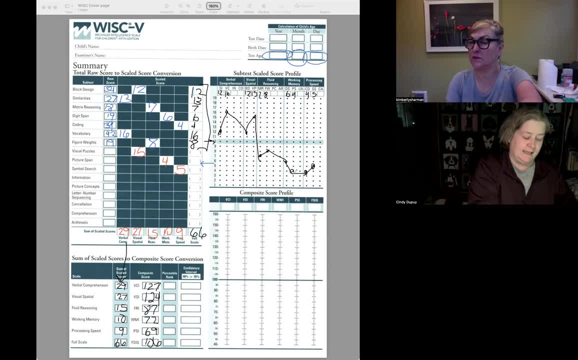 Do most clinicians at school do this? Do they do this little dot thing chart? Some do, some don't, Because this is a big, Very good representation for a parent to see. something is off with this scoring or this testing, Something wacky. So it doesn't have to be that there's something wrong with the testing. 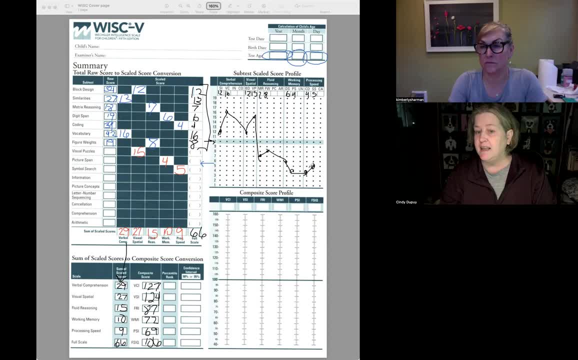 That's true. It can be telling you: hey, your kid has something going on in working memory and processing speed. There is something getting in their way of holding information and working quickly And you, as a parent, need to understand that. What was that? 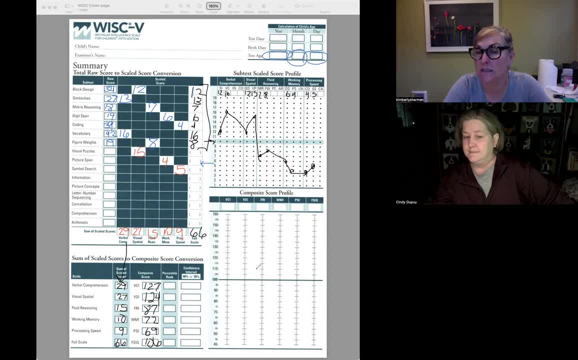 Right. You, as a parent, need to understand what that means. Yeah, He's really skilled in this area, but not in this. There's something going on here Now. similarly, and again, we just made these numbers up, So don't anybody go look up the. 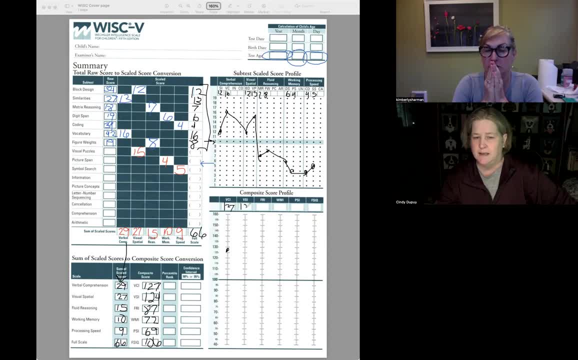 tables and tell me that I've done these wrongs because again I am just randomly making up these numbers. But we're going to look at how the index scores also change as we plug them in over here And then hopefully I haven't overguessed the full scale IQ here. 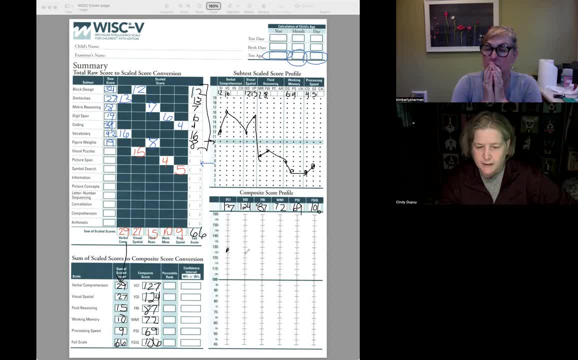 So we've got a 127.. We've got a 124.. We've got an 87 that I've just randomly made up. We've got a 72.. We've got a 69.. And then we've got a 106, which 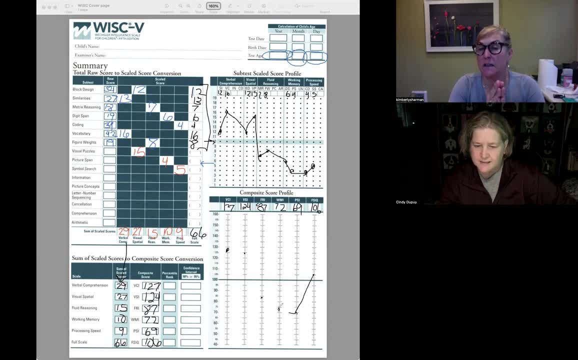 Okay, And these composite scores. the difference between the subtest is, that's within the student himself, but this is compared to the rest of everybody else. his age, Is that right? So the index scores or the subtest scores, are how your student did relative to other students. 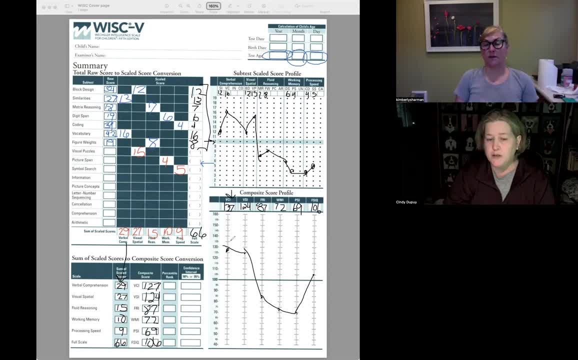 of that age. Okay, When you see this profile of scores jumping all over the place like this, this tells me there is something clearly getting in the way of this student's learning And there's something weird going on. And that's not weird judgmental, That's like this kid does.